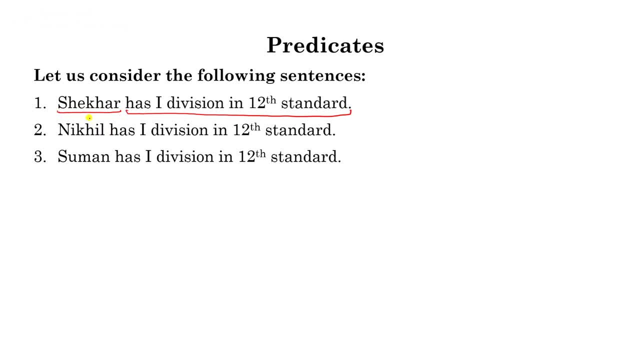 first division in 12th standard. Then the prepositions for each of these students will be: shaker has first division in 12th standard. Second one is: nickel has first division. Third one is 1 and up to 50. So what I will do, I will write, I will denote it, this by P1,. 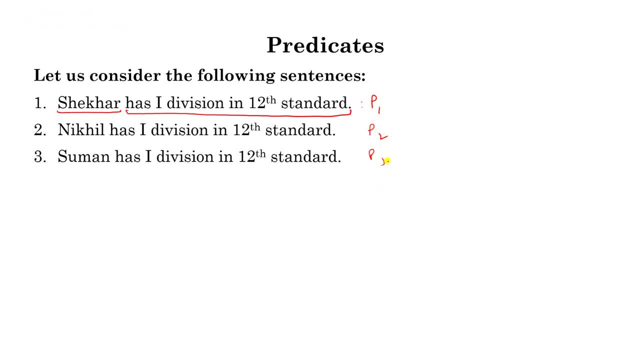 this by P2, P3 and up to so. So for all students have first division means I have to write shaker has first division and nickel has first division, and so on, and so this will be written by P1 and P2 and P3. 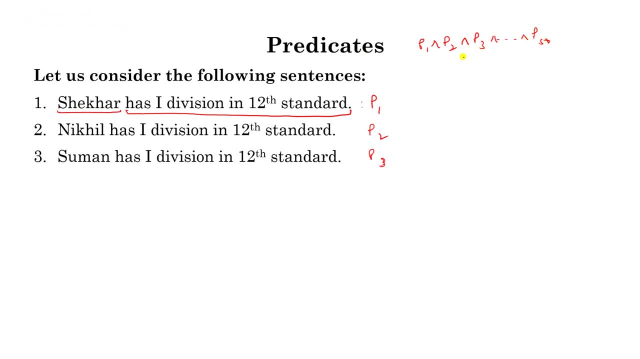 and so on. this is P50.. Now, this is very awkward to write in this way, because if number of students are very large, so this is not a perfect way to write prepositions in this way. So how can we make this process easy Now? 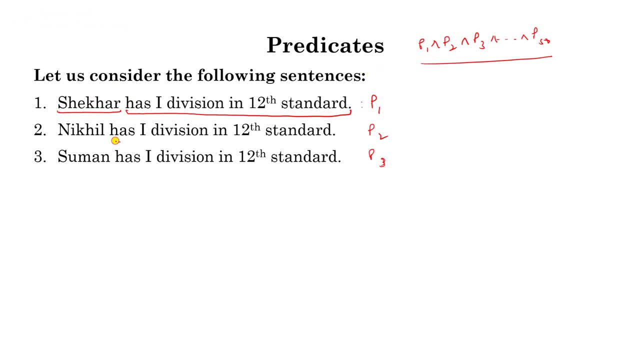 if you look at this, in all these sentences this predicate is common. this predicate is common. So if I write predicate, not in the term of name, but I write if I use a variable x, this is predicate on x, and say: x has, x has first division, first division in 12th. 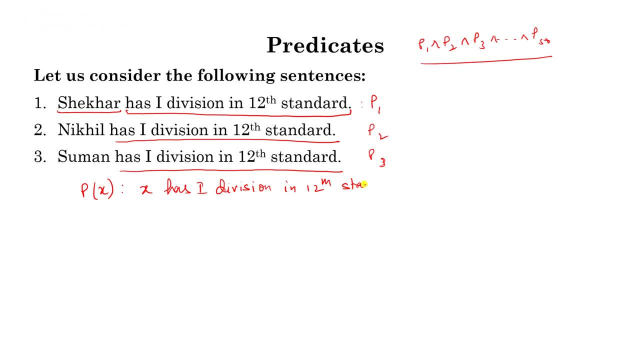 standard. So now, in place of name, I have used a variable, x, and I can define the values of x If we define a set from where x is taking its values. so this set is known as universe of discourse. universe of discourse. 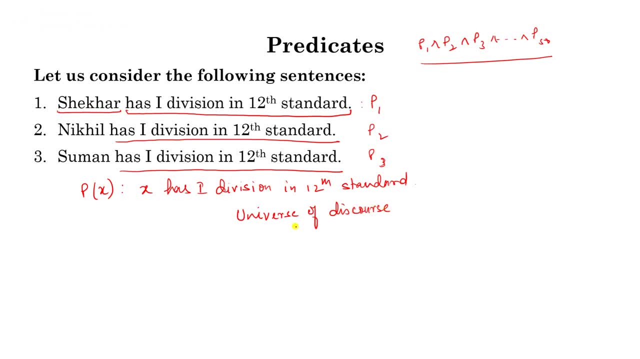 So universe of discourse is the set from where x is taking its values. For example, here you can define: x belongs to set of student, set of students of 12th class, set of student of 12th class. So this is the universe of discourse for x. 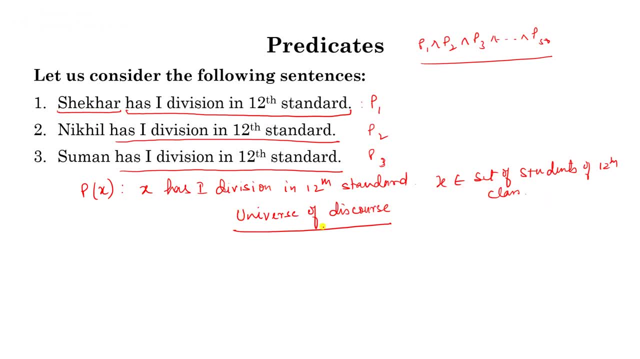 So it is your choice whether to define the universe of discourse for x or not. If you define, then x will take its value from this set. If you do not define universe of discourse, then it can take any value from the universal set. It may be a straight or any other thing. 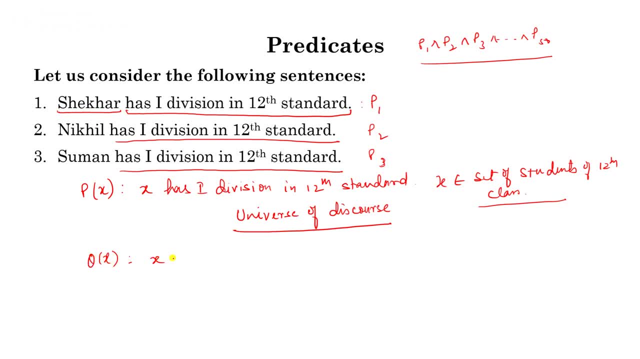 For example, another example: say: if I say qx, x is an even number, x is an even number, x is an even number. So if I define universe of discourse, say x means x belongs to a altogether life condition, Right? So this is these terms. So for rearrangeachntion we need the exact everening of the form empty. 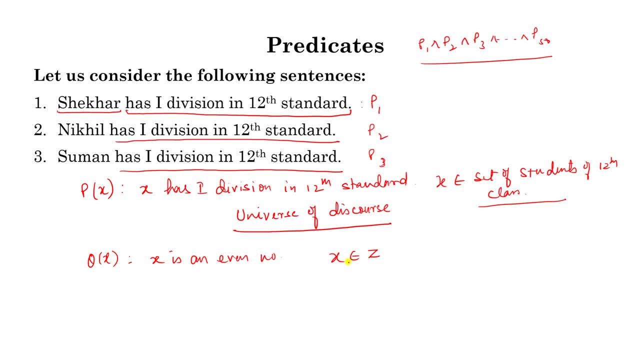 table, And here weters it in the Means to a concrete equation. so one variable, a right is the x belongs to set of integers, then this is the universe of discourse for x. so if i do not define any universe of discourse, then x can take any values, whether it is meaningless or 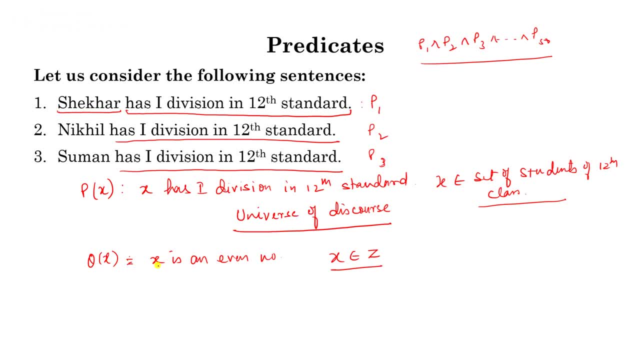 meaningful, but it can take any value if you do not define universe of discourse. universe of discourse, in simple term, you can say the domain, domain of x. so this is the universe of discourse for x and this is your choice: whether to define domain or universe of discourse for a variable or 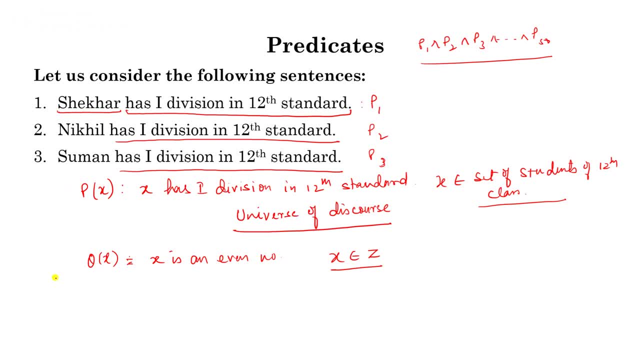 not. so these are predicates on one variables and to write the proportion for the sentence all students have five digit and twelfth sentence. first we will discuss some quantifiers, then we come to the symbolic form of these type of sentences. one thing: these are predicates on one variable. you can write predicate on more than one variable for. 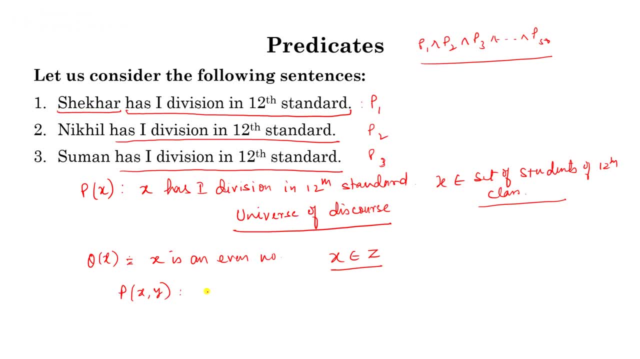 example p, x comma y. so x is greater than y. so there is predicate on two variables, x and y. here you can define x comma y belongs to z. or you can define separate universe of discourse for x and y. so this is your choice. now we will discuss quantifiers, then we'll 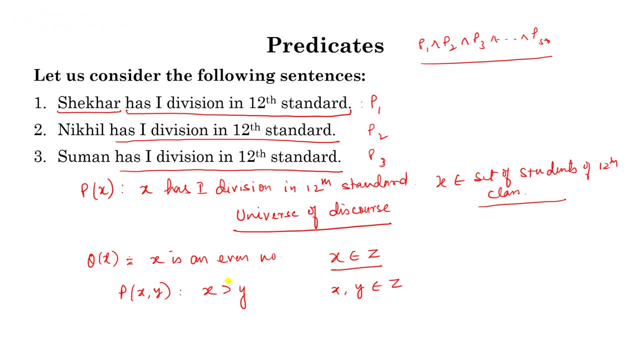 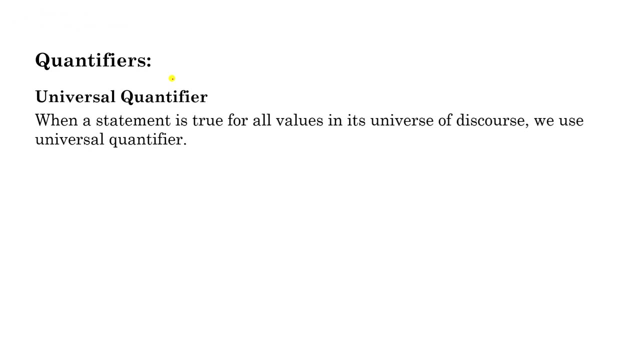 come to how can we define predicates for different types of sentence and how can we write propositions for these type of different types of sentence. quantifiers: quantifier is used to quantify a variable. it means how, for many values, px will be true. 내려 mط cycle. 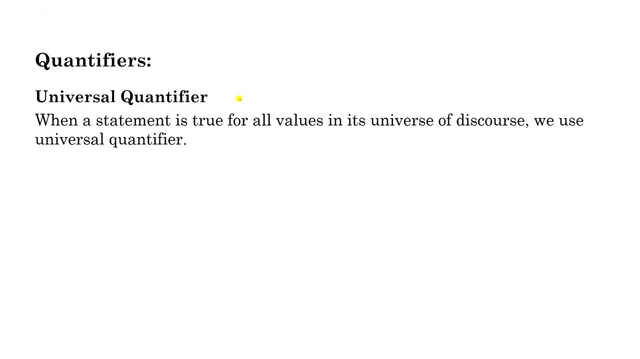 so two types of quantifier are there: are at the side and the bottom and the at the top and 들어. two types of quantifiers are there. one is universal quantifier. here i will discuss universal quantifier, then we will discuss existential quantity. so universal quantifier, when a statement is true. 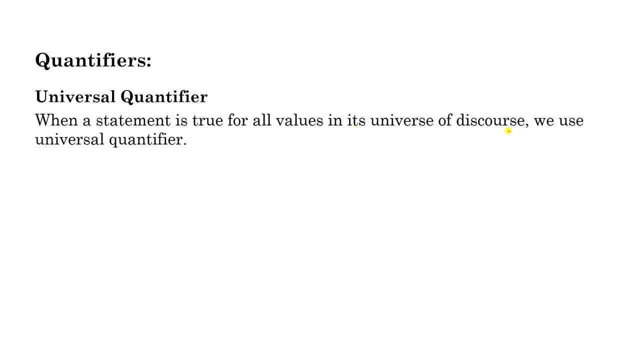 for all values in its universe of discourse or domain, then we use universal quantifier, we use symbol for all or all is for all for you, for this universal quantifier. now look at this, for example: suppose x belongs to the set. 2, 4, 6, 8, 10, say, x belongs to the set and i write a predicate on x. 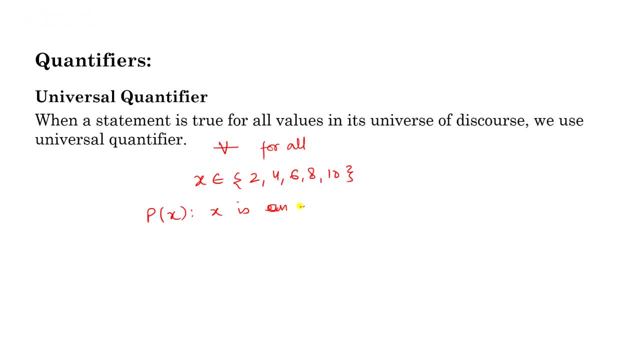 x is. x is an even number, even number. now look at this. this, this sentence, this x is an even number. this is true for all values of x in its universe of discourse. so if i have to write all numbers, all numbers here, suppose this set, say this set is capital x, say this set is capital x. 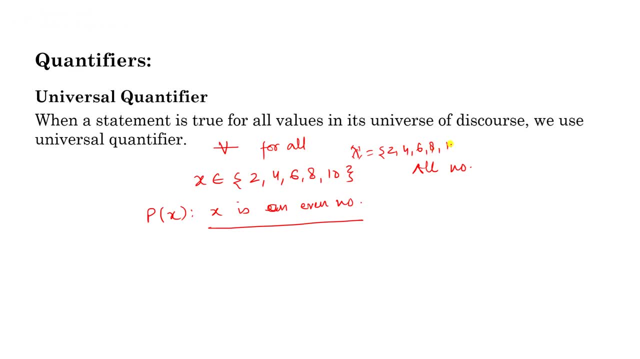 x equal to 2, 4, 5, 6, 4,, 6,, 8, comma 10.. So all numbers in x are even. All numbers in x are even. So the very simple way to write this, because I have written the predicate px, x is an even number. 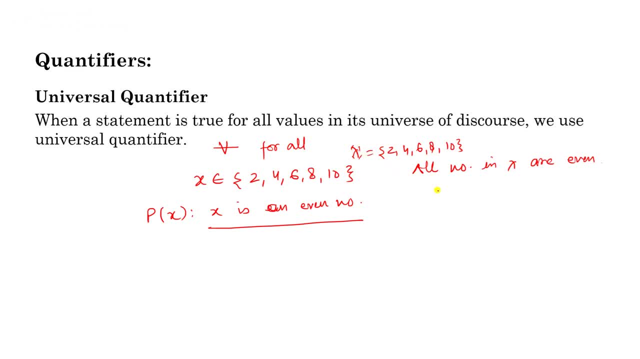 And it is true for all the values in capital X. So how can I write this in the form of this px So I can write it for all x? px Means this is true if px is true for all values of x in its universe of discourse. 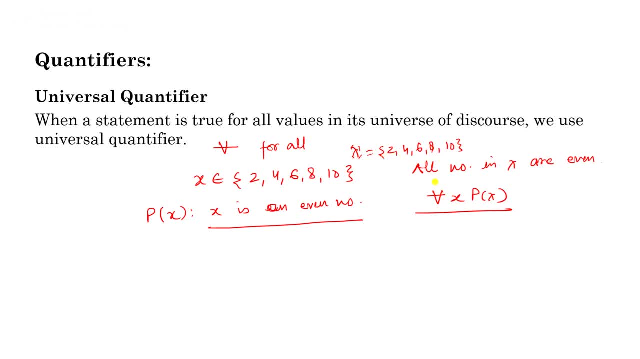 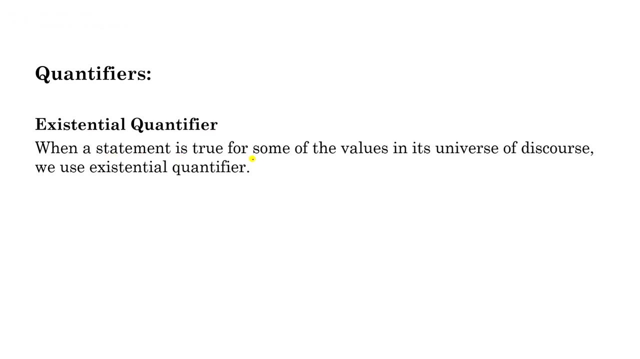 Here it is true: x is an even number for all values of x in its universe of discourse. So we can write it for all x px. Now another quantifier, existential quantifier, When a statement is true for some of the values in its universe of discourse. 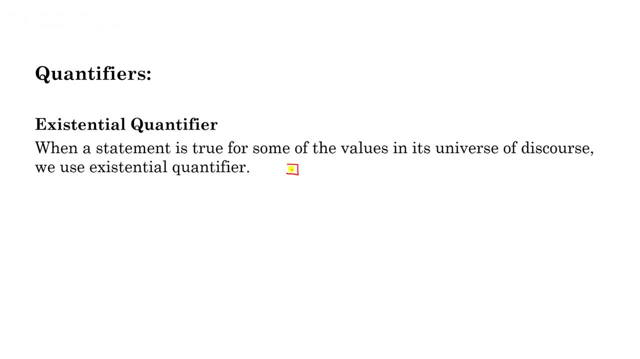 then we use existential quantifier, We use this symbol: there exist, there exist, there exist. Now look at same example again. Suppose x is equal to 1,, 2,, 3,, 4,, 5, 6.. 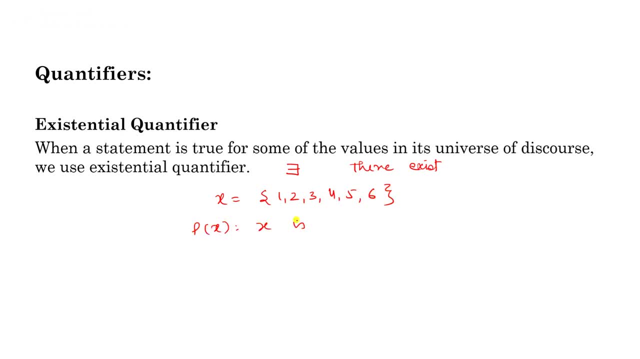 And again, px is, x is an even number, x is an even number. So you know if I write a sentence: some numbers in x, you see this set is capital X. Some numbers in x are even numbers, even numbers. 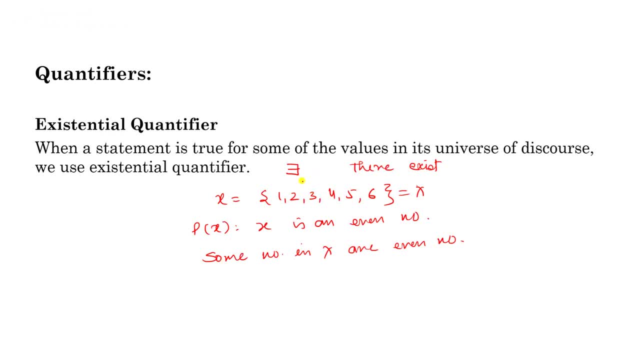 Some numbers. So how can we write it? This there exist. This there exist denotes that some values in the universe of discourse of x are true. So you can write it: there exist x, px. So this symbolic form is for the sentence: some number, some numbers in x are even number. 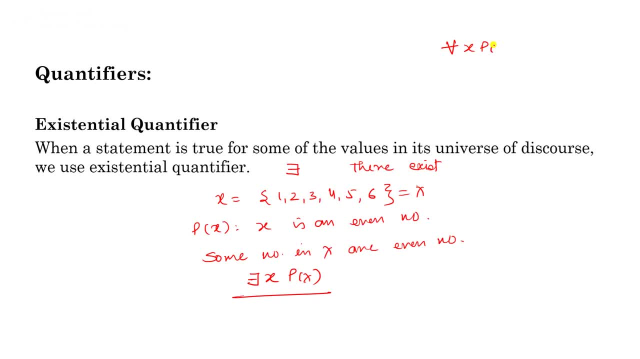 So look at this Whenever we write for all x px. So this will be true if px is true for all values of x in its universe of discourse And false. this will be false if this is false for any one value of one value. 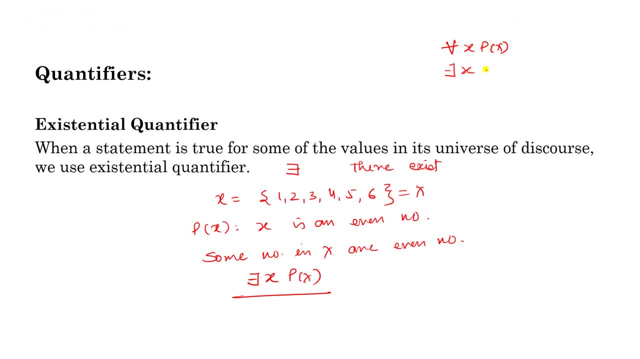 Similarly, there exist x px. There exist x. px is true if there exist at least one value in its universe of discourse for which px is true. If no such value exists for which px is true, then this will be false. And utilizing these two quantifiers for all, x, and there exist x. 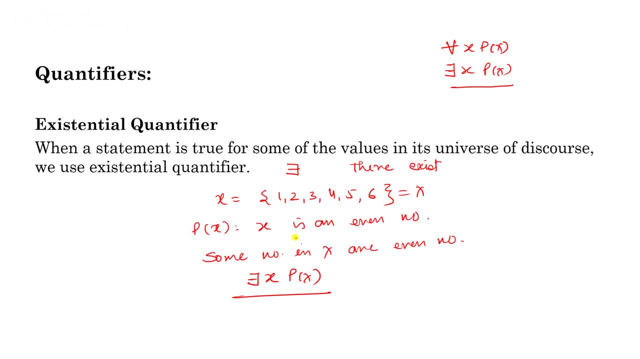 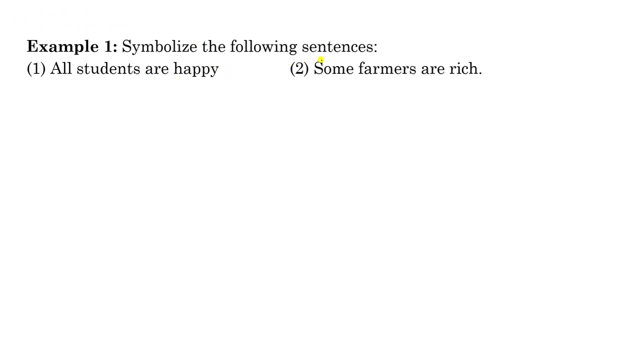 we can write symbolic form of different types of sentences where these types of all, or there exist. these types of words are used. Now here we will consider some examples And we have to symbolize these sentences. All students are happy. 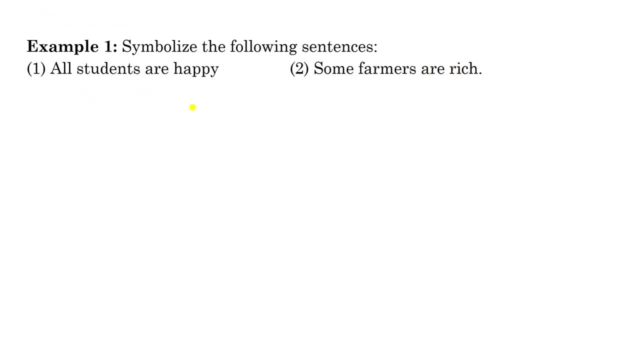 Some farmers are happy. So first we will consider the sentence. We have different ways to symbolize these sentences, So first we will symbolize the sentence with using. with using Universe of discourse, Universe of discourse. So first using universe of discourse. 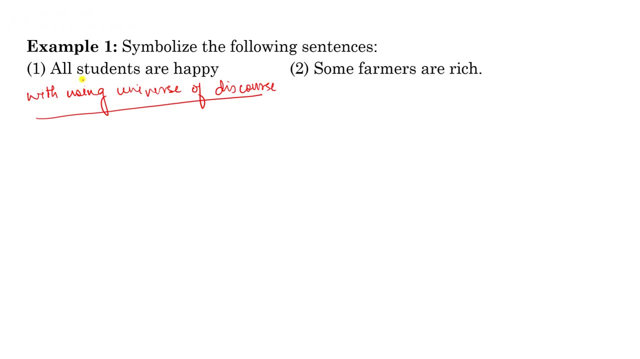 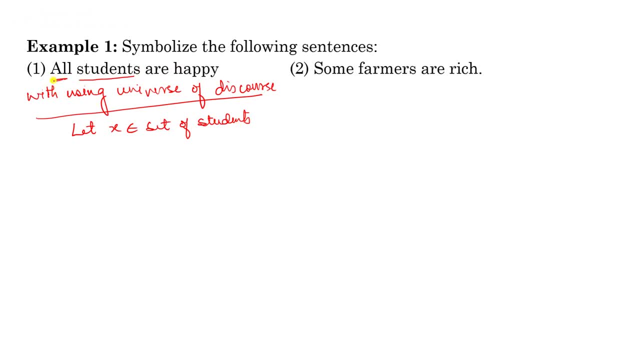 Look at this. All students are happy. This is a quantifier. We have defined the set of universe of discourse for x. Now we can write a predicate on x. x is happy, x is happy. Remember one thing: This part is a predicate on x. 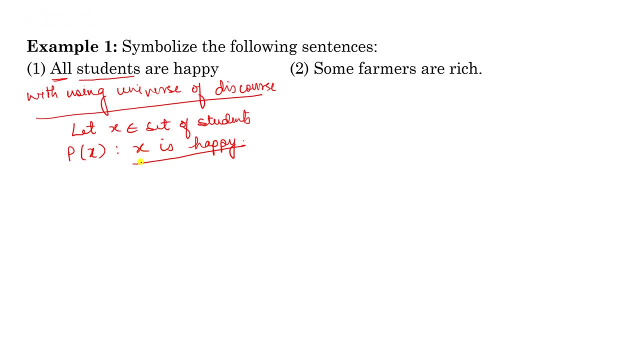 Many times students make a big mistake that they write a predicate but they do not use any variable. Without a variable, this predicate is meaningless. Because you are defining a predicate on x. it means this sentence is telling something about x. If x is not there, this sentence has no meaning. 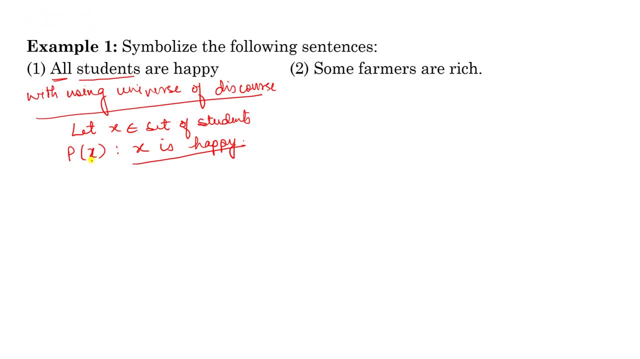 So whenever you define a predicate, you must use a variable. Variables mean more than one, So you have to define something. This part will define something about this variable, So this variable must be there. Without this variable, this is meaningless. 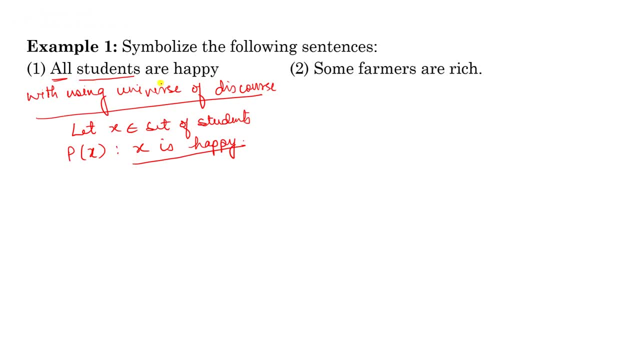 So px is x is happy. Now, for all students are happy. simply, we can write: for all x px, For all x px. So this is the predicate, This is the symbolic form of this student: All students are happy. 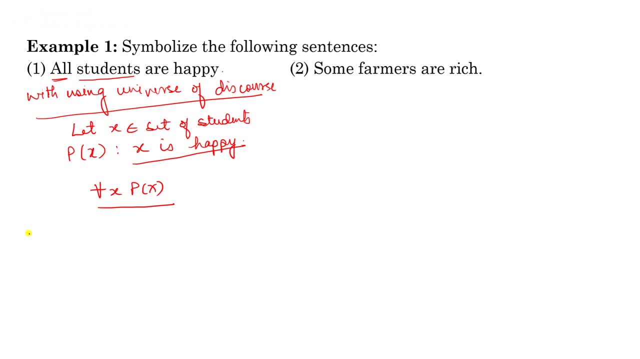 Now second way: Without using universe of discourse, Without Here I write Without universe of discourse, Without universe of discourse. Now look at this Here: if I am not going to define a universe of discourse, it means x can take any values. 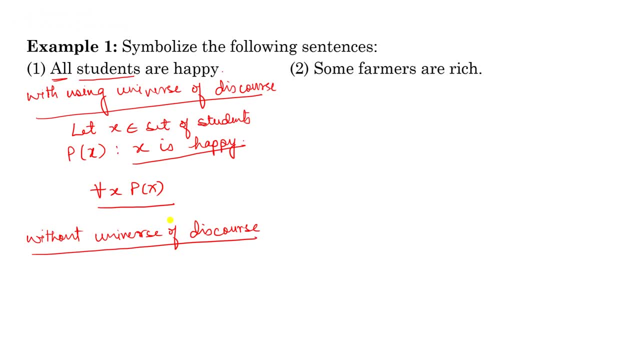 Any values means it may be a student or it may be any value other than a student. So first I have to check All students are happy This is given. It means first I have to check whether x can take any value from the universal set. 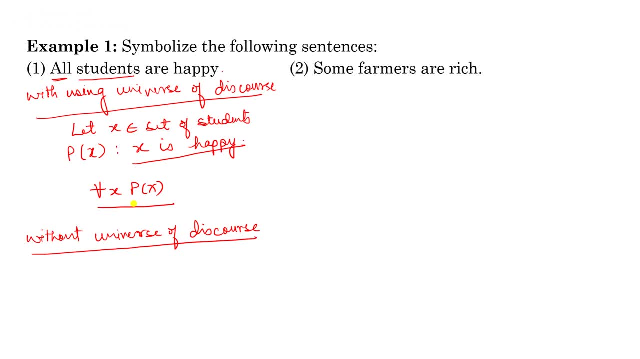 So, whether this value x is a student or not, It means I am using a conditional statement. So I have to define two things. First I will write one predicate for x is a student, x is a student. The second time I will define another predicate: qx. 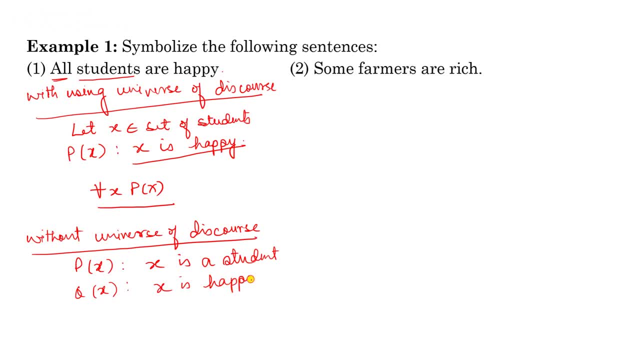 x is happy, So all students are happy. How can I write it For all? x means it can take any value from the universal set, So all students are happy. Universal set: It may be a student or it may not be a student. 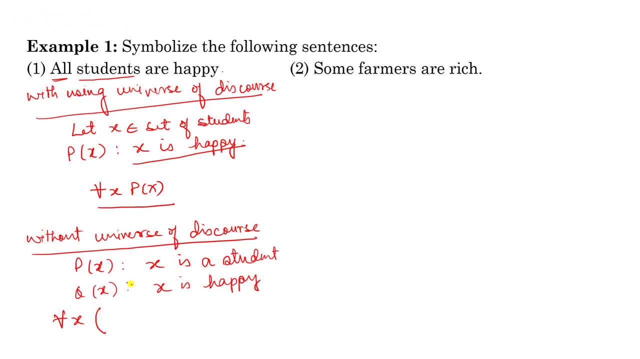 So we are talking about for all x, For all x, But we have to check whether x is a student or not. If it is a student, then it is happy, He or she is happy. So here I am using a conditional statement. 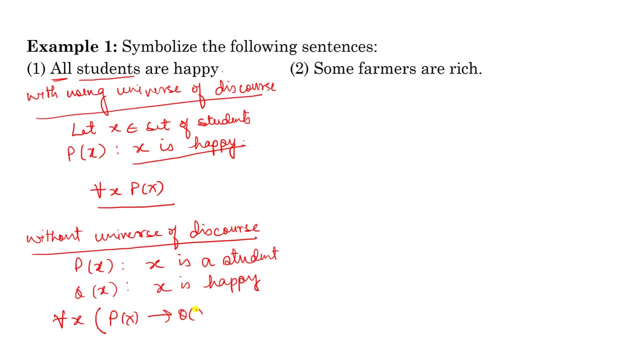 This px implies qx. Look at this: For all x. px implies qx Means for all x, all values of x. If x is happy, If x is a student, then he or she is happy. So this is a symbolic form of this sentence, without using universal discourse. 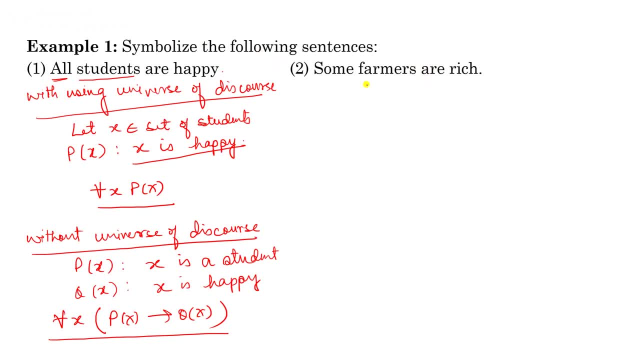 Now look at the second example. Some farmers are rich, So first we will symbolize it using universal discourse. So let x belongs to set of farmers, Set of farmers. Now define px. X is rich, So for this, some farmers are rich. 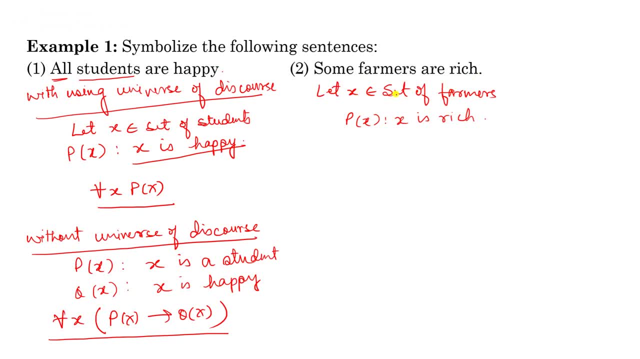 We have already defined universal discourse for x as set of farmers. It means x can take its value from set of farmers. So we can write the symbolic form: as there exists x px, So there exists x. This means for some of the values of this set, x is rich. 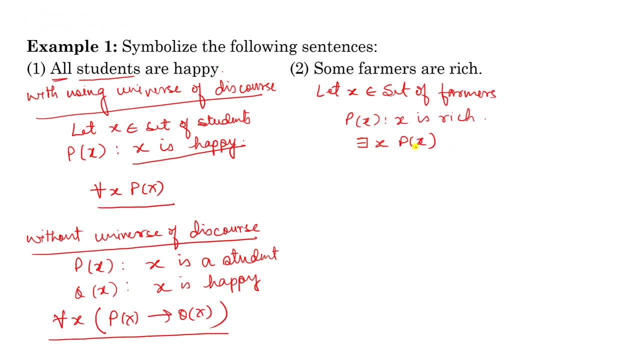 It means some farmers are rich. X can take the values from this set only, So some farmers are rich. Now, second way, without defining universal discourse, What we can do Here? I am not going to define universal discourse. This means x can take any value from the universal set. 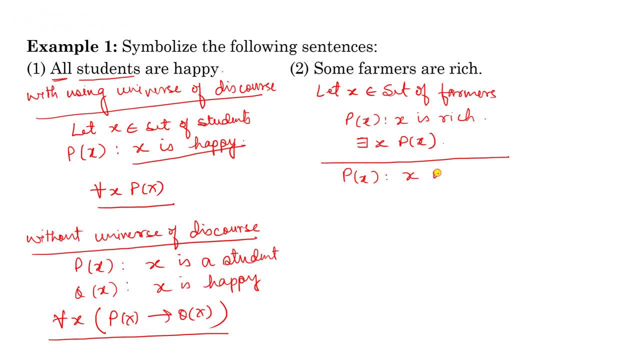 So we will define px, x- x is a farmer, x is a farmer And qx- x is rich. Now how can we write the symbolic form Here? look at this. It is very important to understand this one. 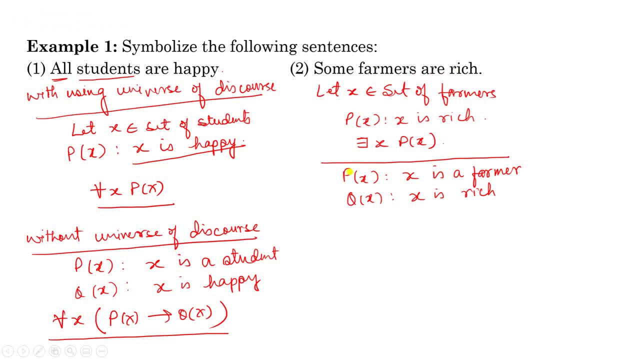 Some farmers are rich. It means some of the values from the universal set are such that they are farmers and rich. I am using and Some farmers are rich. It means some values, Some values are there such that these values are farmers and these values are rich. 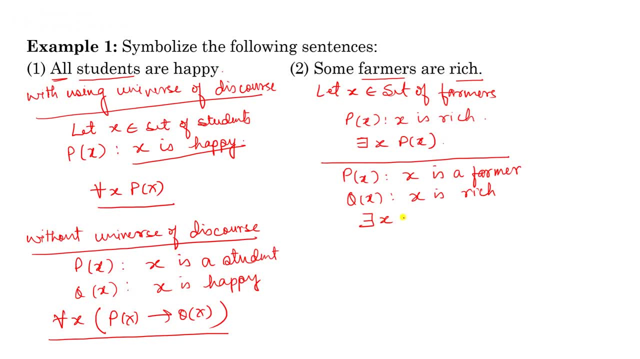 So how can I write it? There exists x, px and qx. There exists x, px and qx means some values of x are there such that they are px and qx. Now you may ask one question, that why we are not writing this. 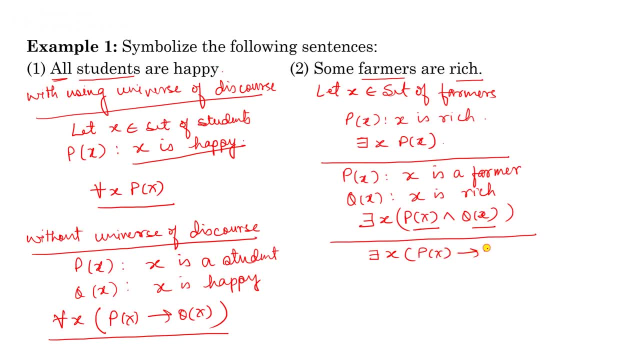 px implies qx, Why we are not writing this in this way. Now look at this. I will give you one example so that it will be clear to you that why we are not using this one for symbolic form of this sentence. If I write, there exists x, px implies qx. 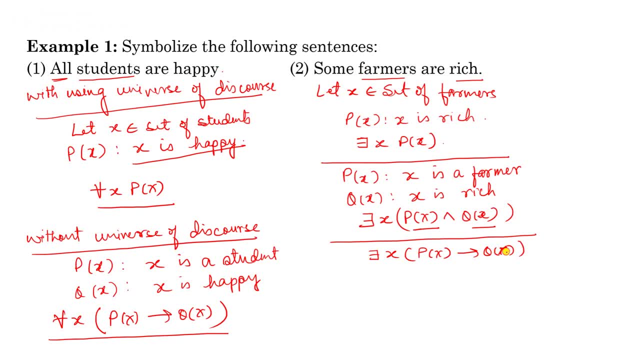 px implies qx, So it means this part is true for some of the values of x, some of the values of x. and say: suppose i say p1 is a person, x say y is a person, y is the name of a person for which this is true there exists. x means 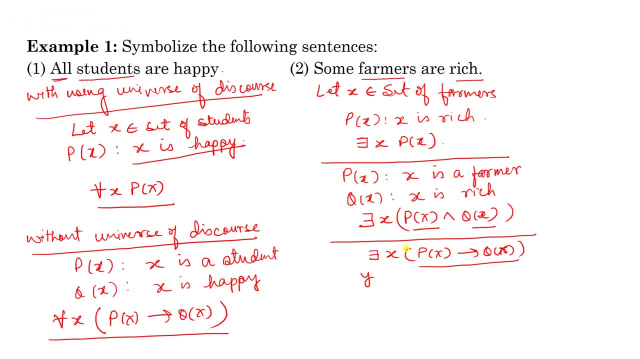 suppose y is a person for which this is true because there exists x. there exists x means a particular value of x exists from a universal set, and suppose this value is y and y is a person. so it is true for y. so if it is true for y, then we can write: py implies q. y means py implies q y. 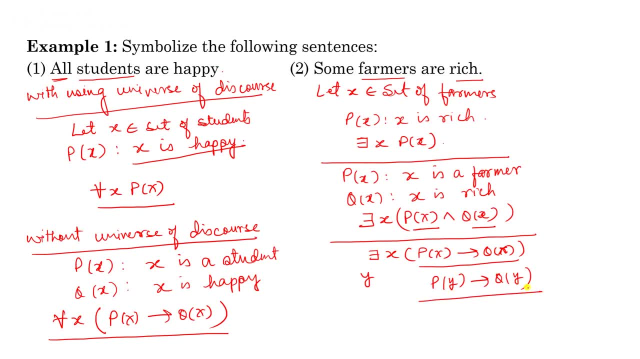 now look at this: this conditional statement may be true if only this part is true. but this part is false means this this: this part is false and this part is true. so this conditional statement will be true if q- this person y is rich, but he is not a farmer. so what we are talking about- some farmers are. 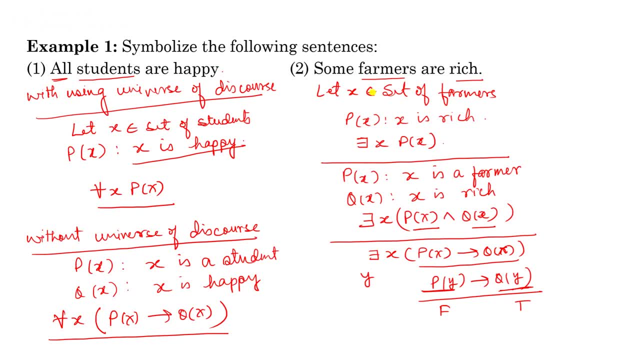 rich means a person or any value which we are taking from universal set. this value is a farmer as well as rich, and if we write this symbolic form in this way, so this will be true in this way. so this will be true in the case where this y is true, but this q, this, this part is true, but 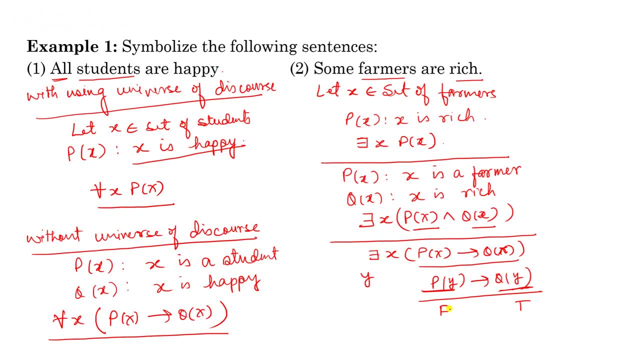 this p? y. this part is false. it means these two conditions farmers, and these both are not satisfied. that's why we cannot write the symbolic form in this way. so for these type of sentences- some farmers are rich. we will write: there exists x, px and qx. it simply means some value is not satisfied. 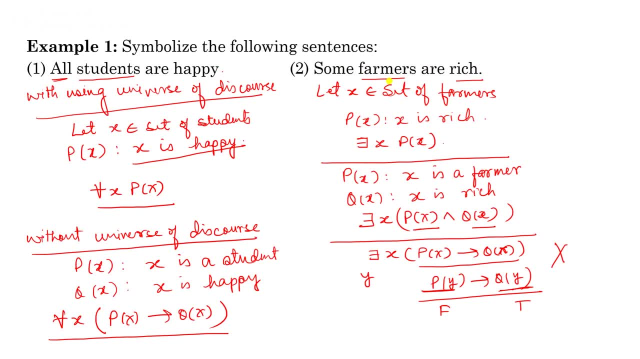 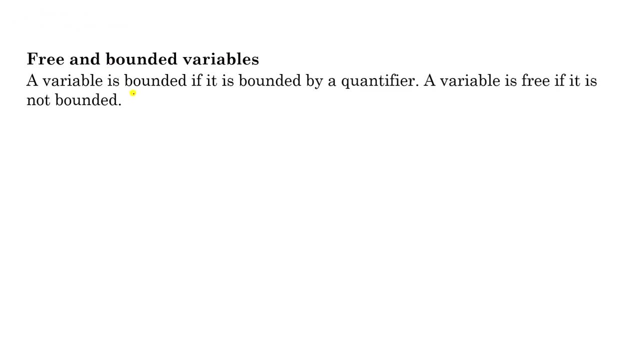 values of x are there such that x is px and x is qx. Now free and bounded variables. A variable is bounded if it is bounded by a quantifier. A variable is free if it is not bounded. For example, suppose, if I write for all x, pxy, Suppose pxy is a predicate on two variables, x and y. So if you 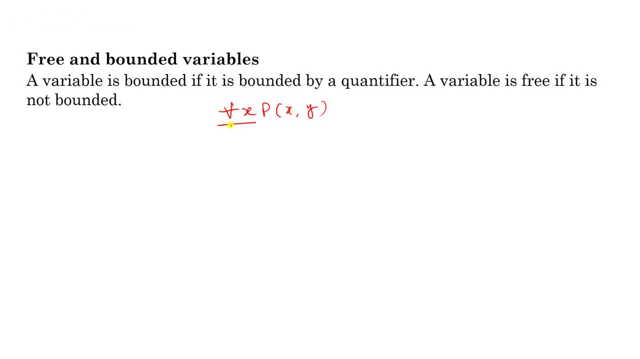 look at this: x for x, we have used a quantifier for all. x means x is bounded by a quantifier, but y is not bounded by a quantifier. So here, x is a free variable, x is a bounded variable, while y is a free variable. Now removing quantifiers from the predicate, 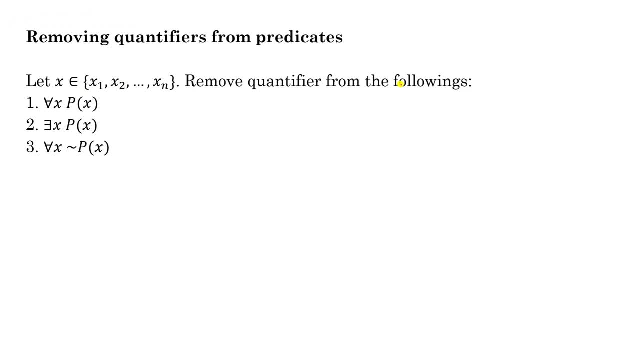 Look at this. suppose x belongs to x1, x2, xn. Now we have to remove the quantifiers from this for all x px. So whenever we write for all x px, this is written in the form of this predicate: px means px is true for all values of x given in its universe of discourse. So we have, if we have, to remove. 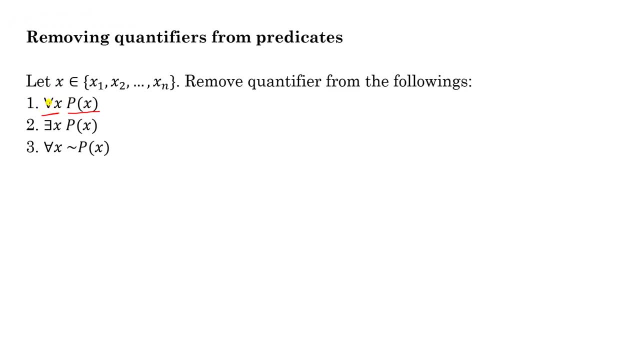 this quantifier. it simply means we have to write these prepositions for each of these values. So here, for all x. px means px is true for all x. So we can write: if we remove the quantifier, then we will use These prepositions for each of these values, So we can write it px1 and px2 and up to so on pxn, as I 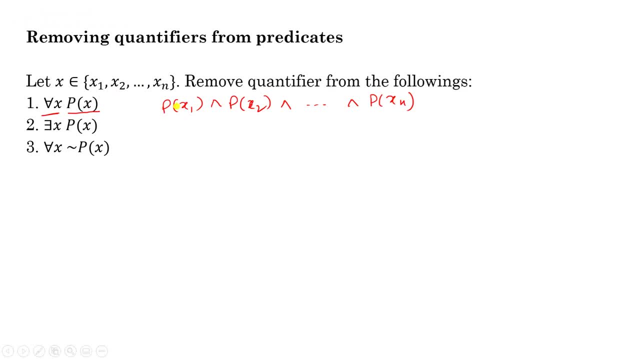 told you in the first slide why we use predicates. So if we remove, we are just basically we are doing the reverse procedure. If we have to remove the quantifiers, it means we have to write prepositions for all these values in its universe of discourse. Similarly, for this one, there exists xpx. 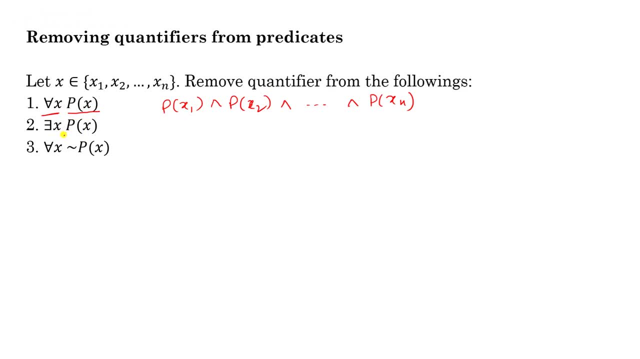 px means px is true for some of the values. of x means this can be written as px1 or px2, or, and up to pxn. Similarly for all x. negation of px- Now negation of px- is itself one predicate. It means: 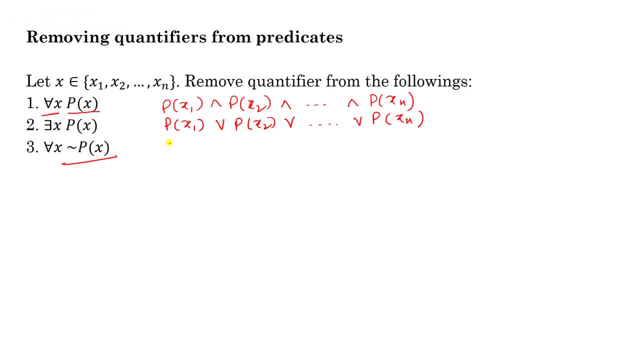 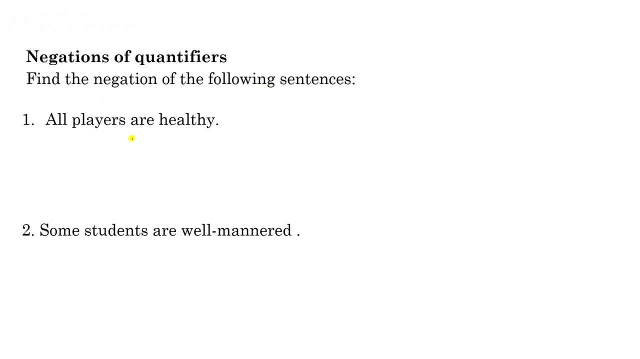 negation of px is true for all values of x. So we will write negation of px1 and negation of px2 and up to negation of px. So in this way we can remove quantifiers from predicates. Now, negation of quantifiers. Find the negation of this following sentence: all players are. 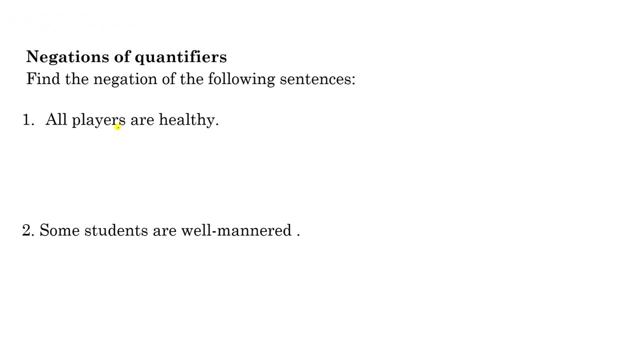 heavy. So to find the negation of these type of sentences, First try to write in symbolic form and then write the negation of px1 and px2.. just i will give you one example. how can we write the negation of sentence, for example, suppose we 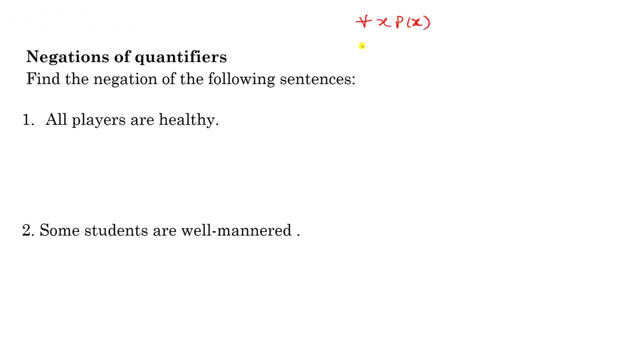 have for all x px, for all x px. so if i write the negation of px, then this will: this is equivalent to negation of: for all x, there exist x, and then we'll write the negation of px. negation of px, it means negation of: this is for all x px. is there exist x. negation of px. similarly, negation of: 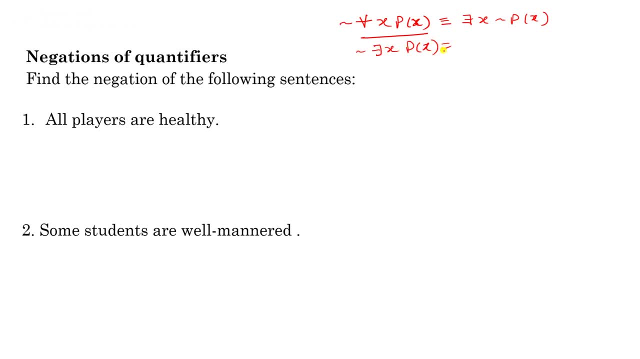 there exist x px. this is for all x. negation of px. so first we will symbolize these sentences, then it will be very easy for you to write the negation. all players are healthy. all players are healthy- suppose i use the universe of discourse- say x belongs to set of players, set of players. 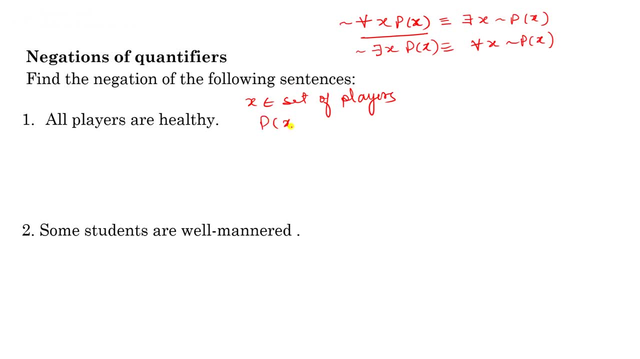 and px. you write px, x is healthy, x is healthy, so you can write for all x px. now, if you negate, this means a negation. this is negation of for all x px. this will be equivalent to there exist x. negation of px. it means some players are not healthy. so negation will be some players, some players. 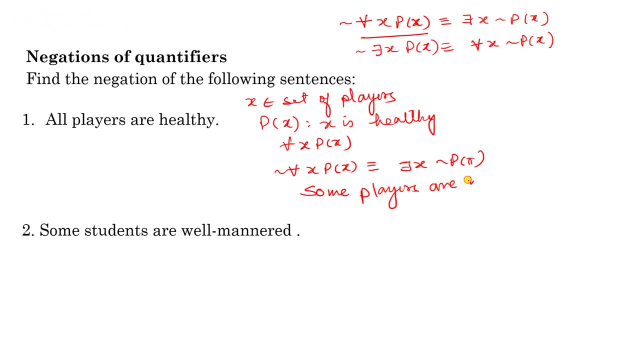 are not healthy. so this is the negation of all players are happy. first, what we did? we simply we have written the symbolic form. then we find the negation of this symbolic form and interpreted the symbolic form in form of sentence. similarly, in the same way, some students are well mannered. here you can write x, x are healthy. 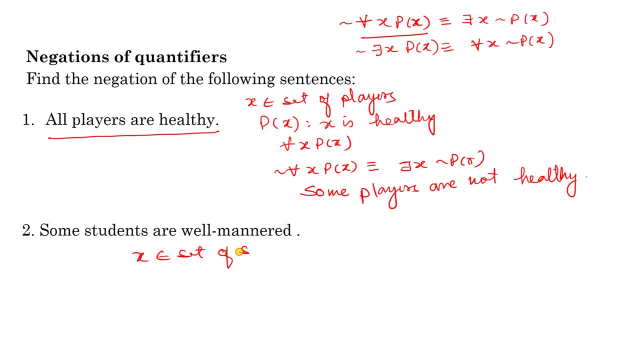 belongs to set of students. set of students and say px, x is well-mannered, well-mannered. so some students are well-mannered and you can write: there exist x, p, x. so if i have to find the negation of this, i will write negation of there exist x, px, and this is equivalent to: